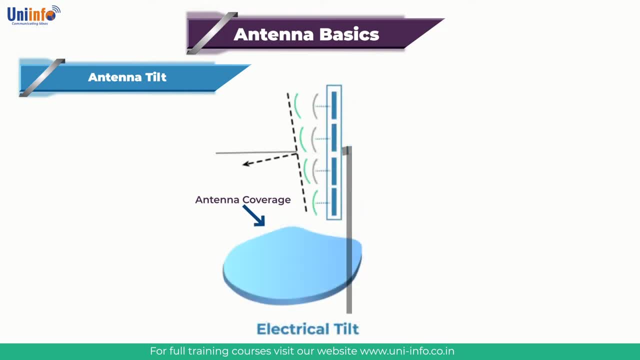 To counter these unplanned side effects, electrical tilting is more commonly used as it provides a consistent horizontal radiation pattern. with the added benefit of a horizontal radiation pattern, A combination of mechanical up tilt and electrical down tilt is occasionally used in problematic areas to provide a conventional main beam, but with down tilt, side and back lobes. 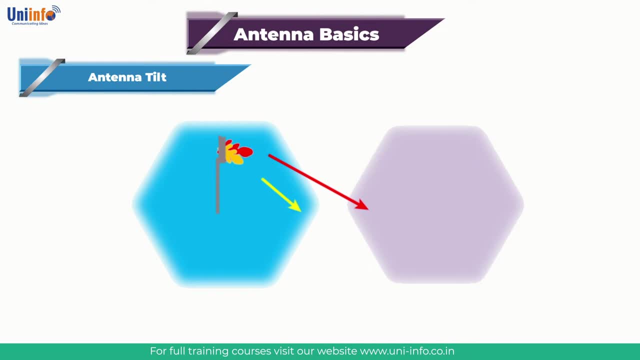 The efficiency of a cellular network depends on its correct configuration and adjustments of radiant systems. They transmit and receive antennas, And one of the more important system optimization task is based on correctly adjusting tilts or the inclination of the antenna in relation to an axis. With the tilt we direct irradiation further down or higher, concentrating. 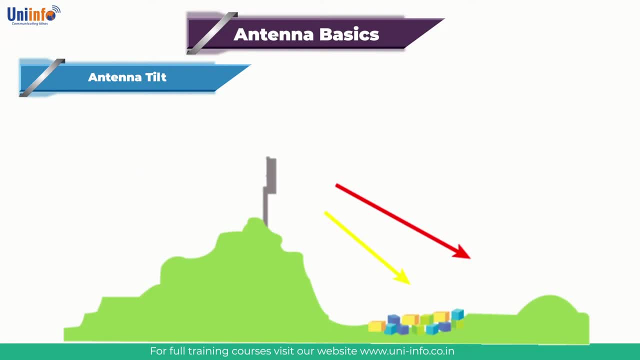 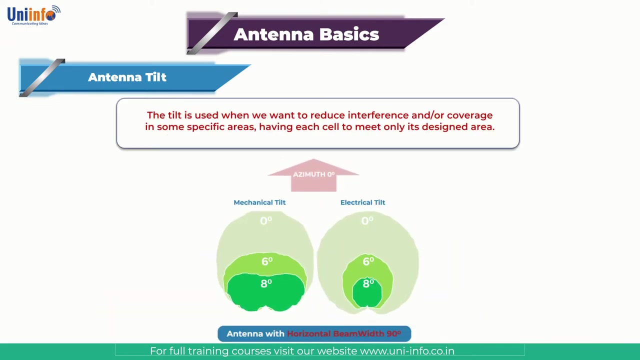 the energy in the new desired direction. When the network is tilted down, we call it down tilt, which is the most common use If the inclination is up- very rare and extreme cases- we call it up tilt. The tilt is used when we want to reduce interference and or coverage in some specific areas, having 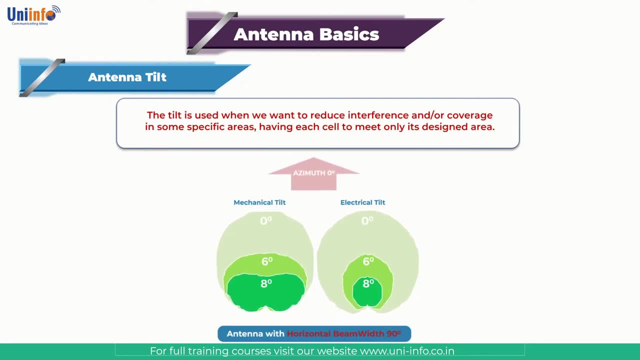 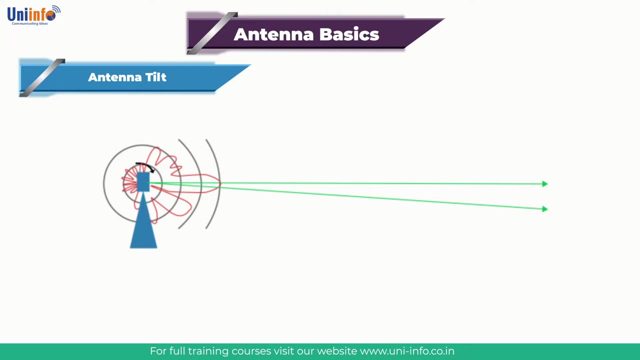 each cell to meet only its designed area. Although this is a complex issue, let's try to understand a simple way how all of this works. Let us understand what is a tilt. Right now we can talk specifically about tilt. Let us start reminding what is the tilt of a cell. Let us start reminding what is the tilt of. 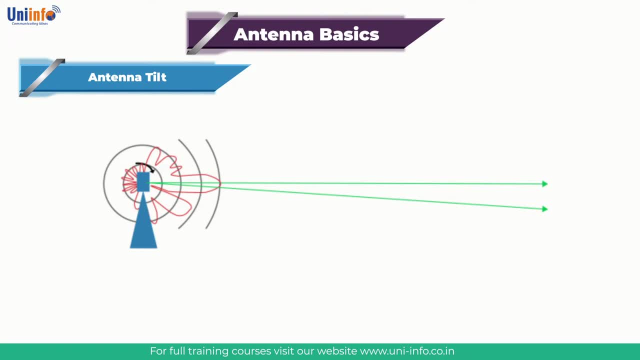 an antenna and what is its purpose. The tilt represents the inclination or angle of the antenna to its axis. We have seen, when we apply a tilt we change the antenna radiation diagram. For a standard antenna without tilt, the diagram is formed as we see in the figure. 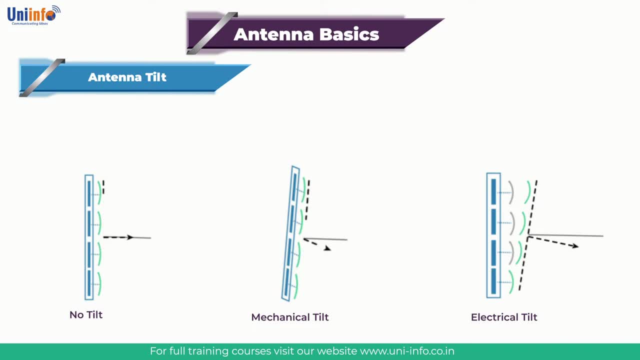 on the screen. There are two possible types of tilt which can be applied together: the electrical tilt and mechanical tilt. The mechanical tilt is very easy to be understood: Tilting the antenna through specific accessories on its bracket without changing the phase of the input signal, the diagram and consequently, 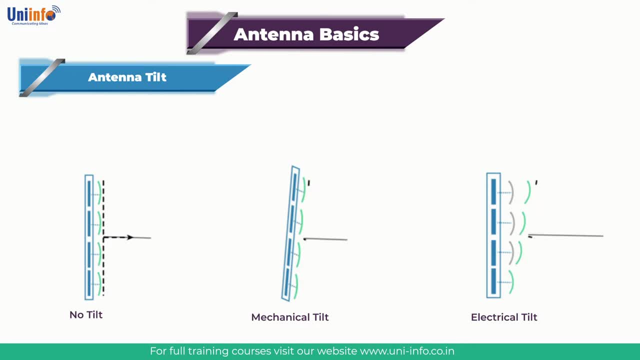 the signal propagation direction is modified And for the electrical tilt, the modification of the diagram is obtained by changing the characteristics of signal phase of each element of the antenna. the electrical tilt can have a fixed value or can be variable, usually adjusted through an accessory such as a rod or bolt with markings. 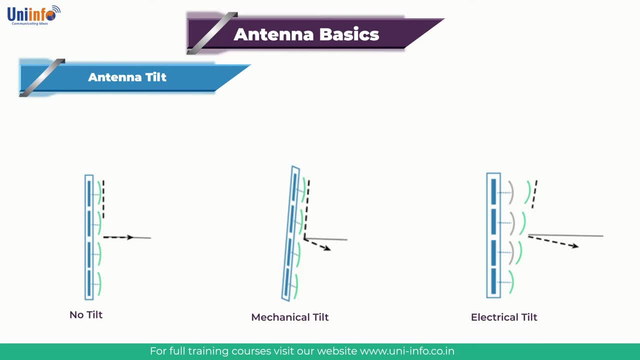 This adjustment can be either manual or remote, In the latter case being known as RET, usually a small engine connected to a screw, stem or regulator that does the job of adjusting the tilt. With no doubt, the best option is to use antenna with variable electrical tilt and 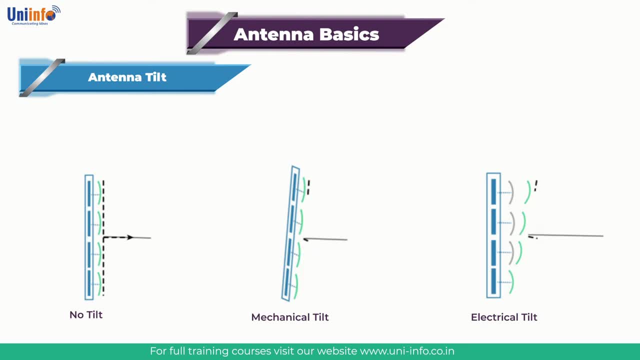 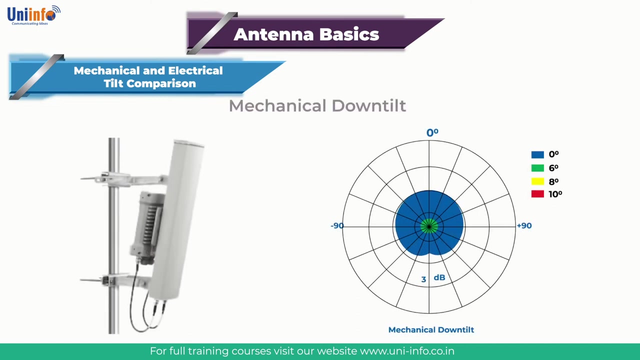 remote adjustment possibility because it gives much more flexibility and ease to the optimizer. However, these solutions are usually more expensive and therefore the antennas with manual variable electrical tilt option are more common. Next topic is Mechanical and Electrical Tilt Comparison. Mechanical tilt is a very common option. 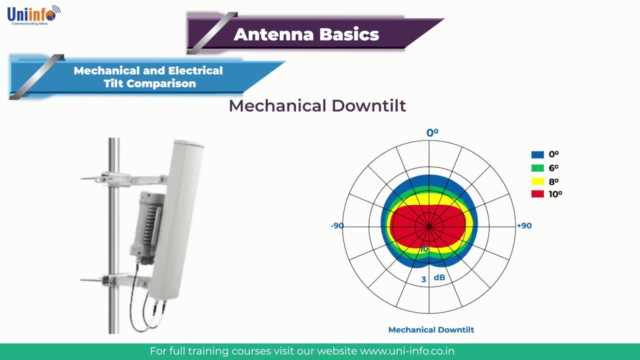 Mechanical down-tilt consists of physically rotating an antenna downward about an axis from its vertical position. In a mechanical down-tilt, as the front lobe moves downwards, the back lobe moves upwards. This is one of the potential drawbacks as compared to the electrical down-tilt, because 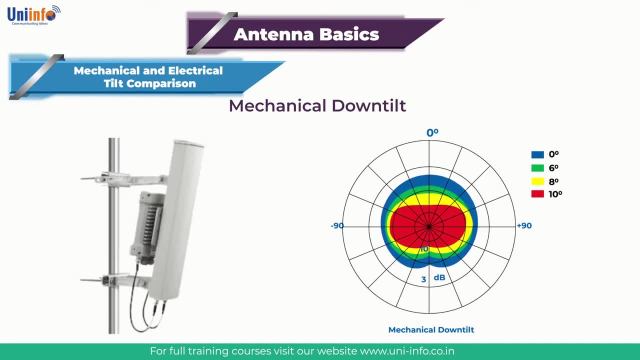 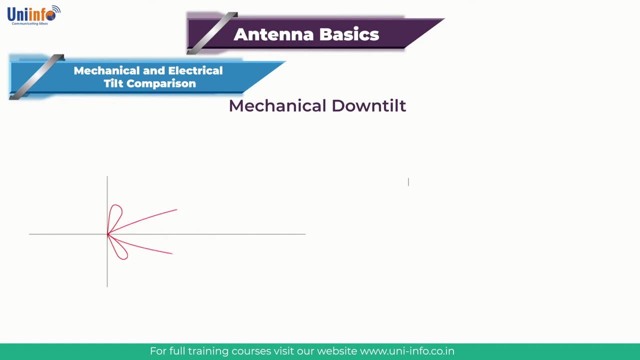 coverage behind the antenna can be negatively affected as the back lobe rises above the horizon. Additionally, the mechanical tilt is a very common option. The mechanical tilt is a very common option as compared to the electrical down-tilt. Mechanical down-tilt does not change the gain of the antenna at plus or minus 90 degree. 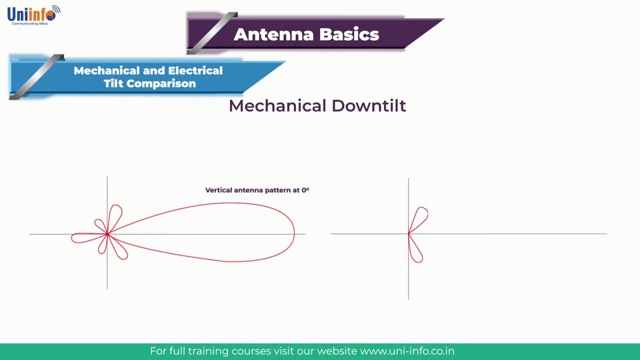 from antenna horizon. As the antenna is given down-tilt, the footprint starts changing, with a notch being formed in the front while it spreads on the sides. After 10 degrees down-tilt, the notch effect is quite visible and the spread on the sides 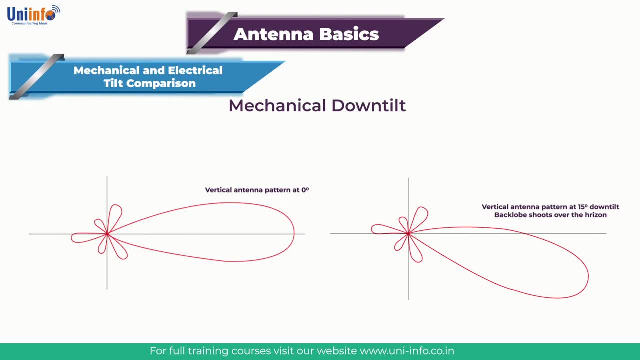 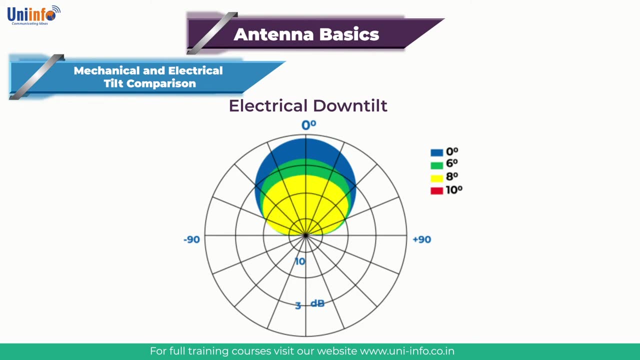 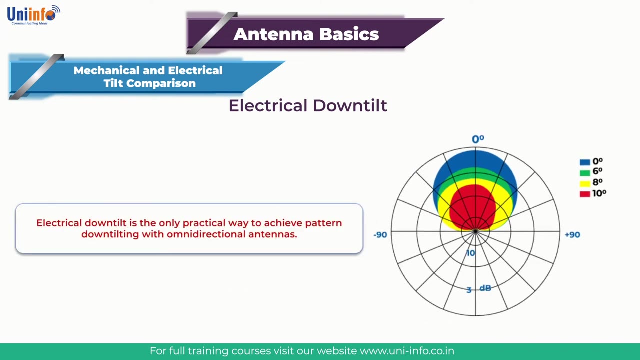 are high. This may lead to interference on the sides. Electrical tilt is a very common option. Electrical down-tilt uses a face taper in the antenna area to angle the pattern downwards. This allows the antenna to be mounted vertically. Electrical down-tilt is the only practical way to achieve pattern down-tilting with the 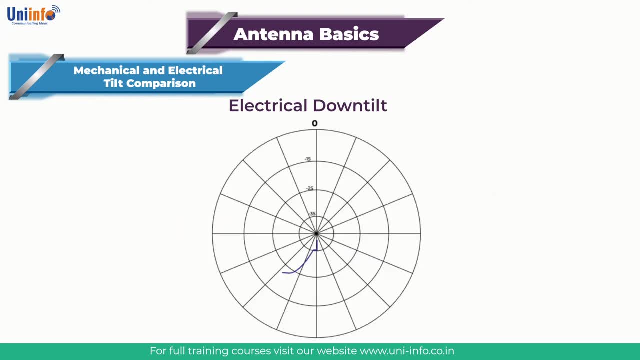 omnidirectional antennas. Electrical down-tilt affects both front and back lobes. If the front lobe is down-tilted, the back lobe is also down-tilted by equal amount. Electrical down-tilt is a very common option. 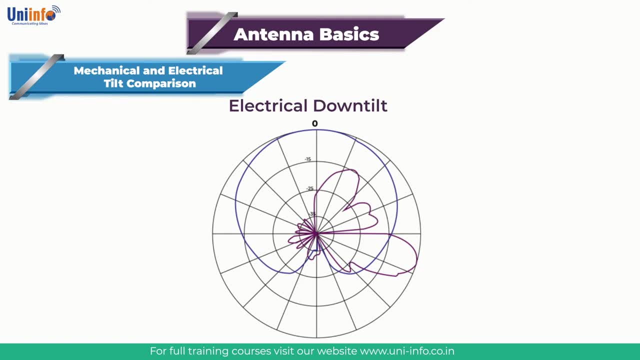 Electrical down-tilt is a very common option. Electrical down-tilt is a very common option. Electrical down-tilt also reduces the gain equally at all angles on the horizon. That adjusted down-tilt angle is constant over the whole azimuth range. 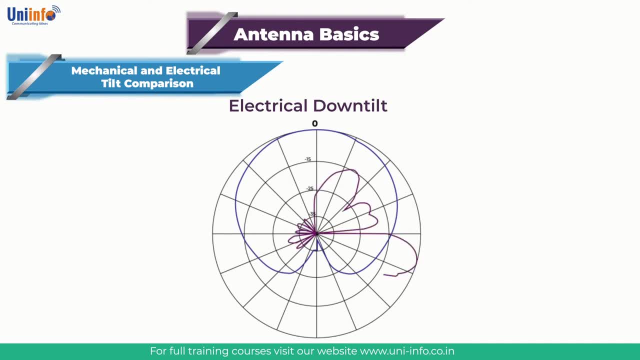 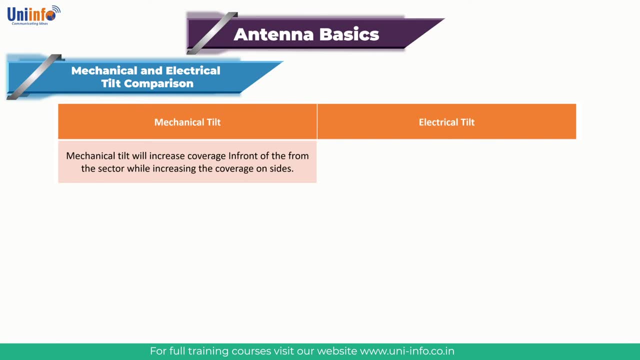 Variable Electrical down-Tilt antennas are very costly. So we can see in this mechanical tilt will increase coverage in front of the form sector while increasing the coverage on sides. While electrical tilt decrease both length and width Like a separator, Soermat이라는 price will decrease. 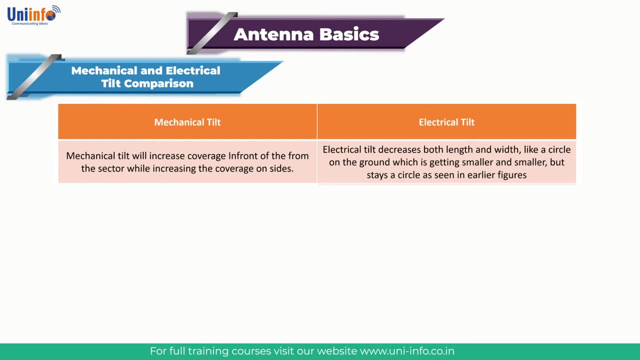 circle on the ground which is getting smaller and smaller but stays a circle, as seen in earlier figures on the screen. Mechanical tilt is used on tall sites, typically on top of hills, because electrical tilt is not enough. The electrical tilt is recommended for sites which are not tall and inside city limits. 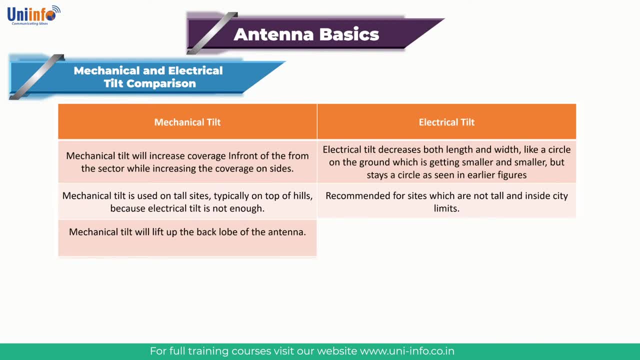 Electrical tilt decreases coverages and adds interference as down tilting of main lobe results into up tilt of the back lobe, and electrical tilt decreases coverage and does not add interference as the back lobe also gets down tilted electrically. In mechanical tilt sector overlaps are increased and in electrical tilt sector overlaps are. 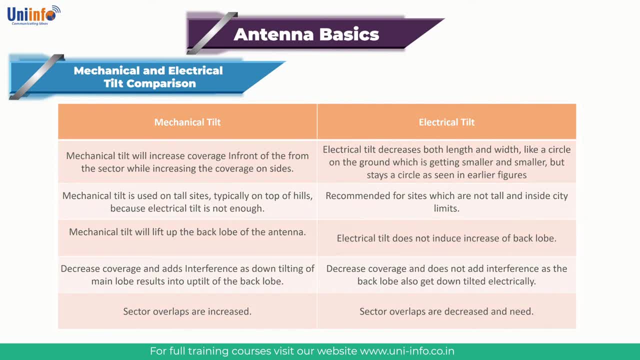 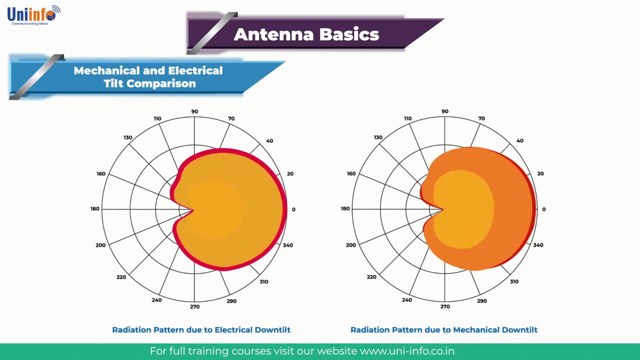 decreased and neat. Now let us understand what is mechanical tilt. Let us understand the major difference between mechanical tilt and electrical tilt. Here the figure on the screen shows the difference between mechanical tilt and electrical tilt with respect to radiation pattern. As shown in the figure, mechanical tilt results into pattern blooming, resulting into a notch. 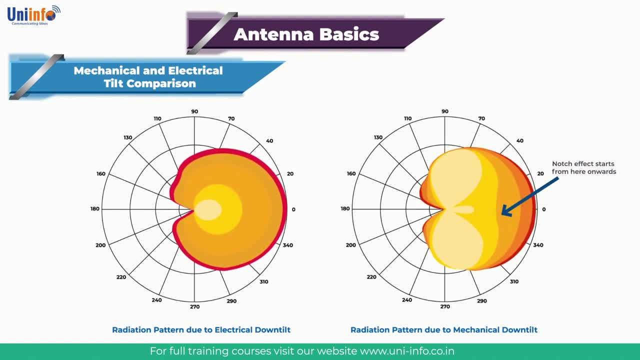 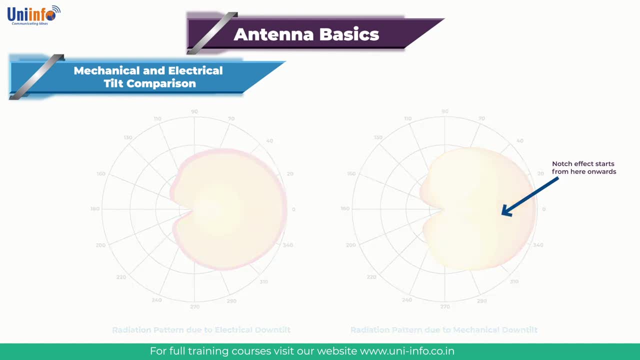 effect in front of lobe of antenna. as the tilt increases with electrical tilt suppresses the pattern bloom. The electrical tilt achieves this result As it is able to tune individual radiating elements of antenna array. Mechanical tilt fails as it tunes the entire antenna as a fixed single unit.